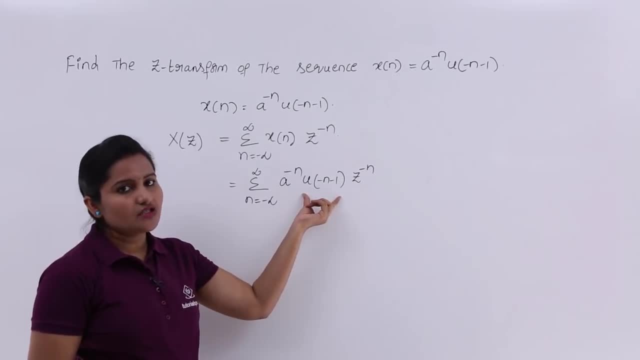 that will change the limits. So now, here also, we are having a unit step function. This is also going to change the limits of this summation. How it is going to change means accordingly to that unit step function. you are going to change. That means wherever the places you are having. 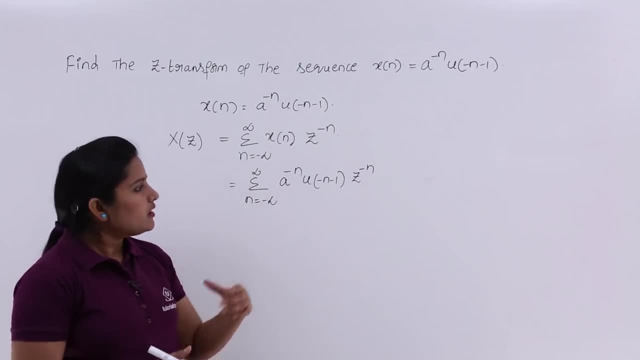 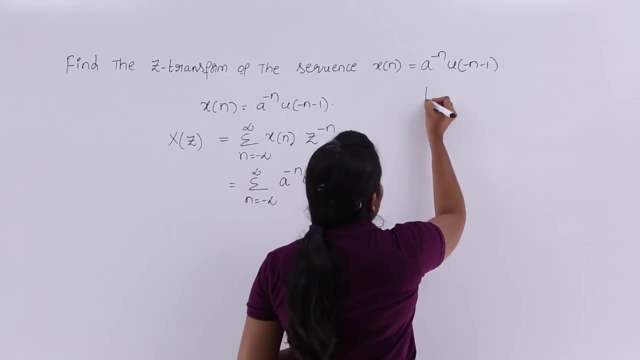 that unit step function. there only you are going to calculate that summation. So what is the region of this unit step function? Generally you are discovery specialization. your discrete unit step- general discrete unit step- starts from 0 and it will keep on extending. 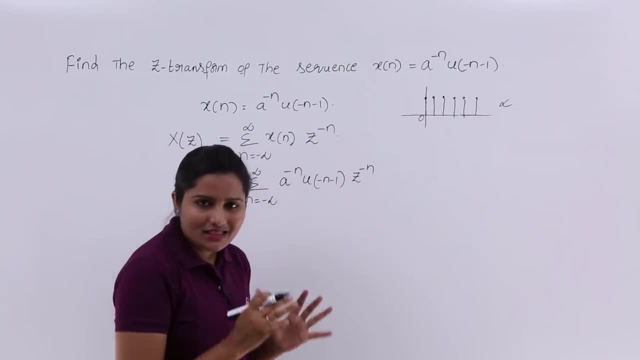 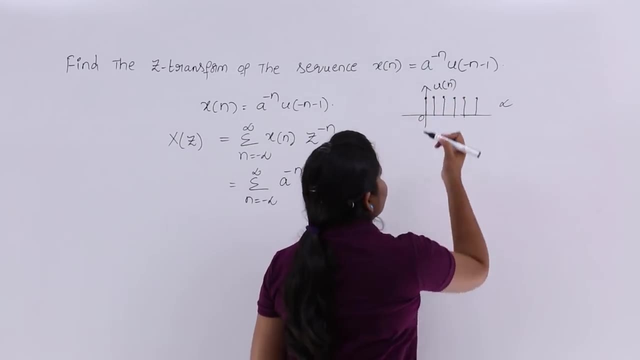 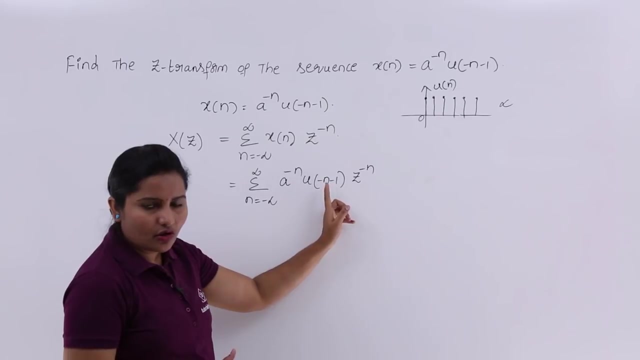 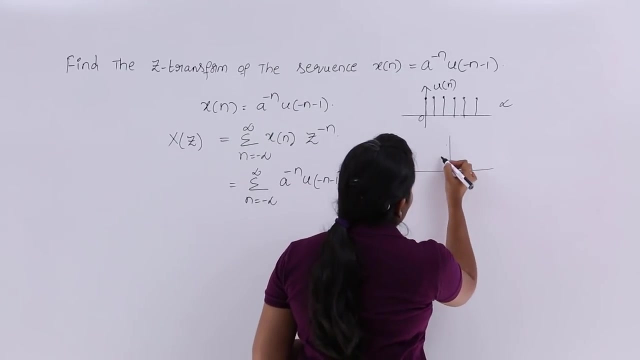 up to infinity, that is, from 0 to infinity. your general unit step, discrete unit step, is 0 to infinity. this is u of n. then what is u of minus n? you just forget about this- minus 1. I will talk about this later. so if this is u of n, your u of minus n will be like: 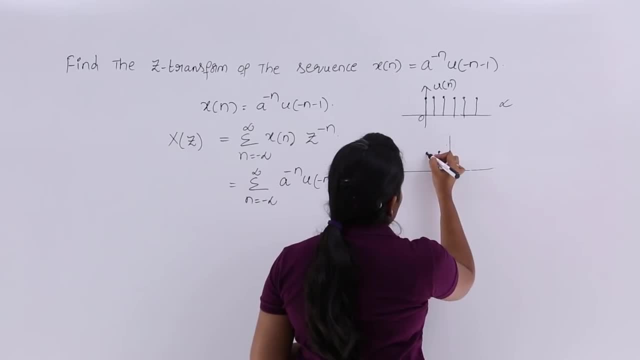 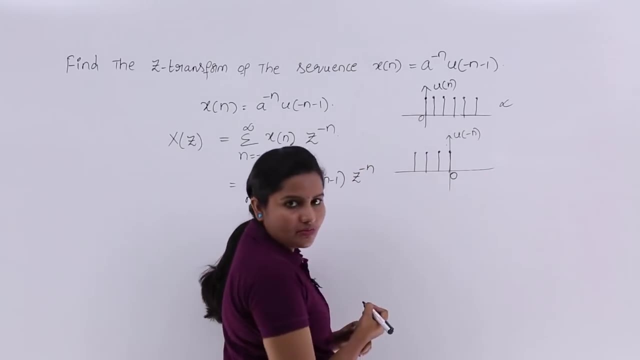 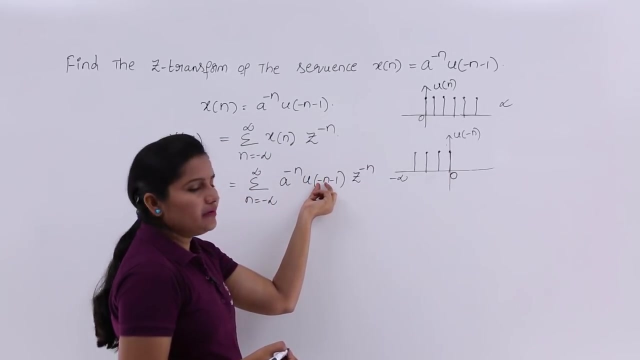 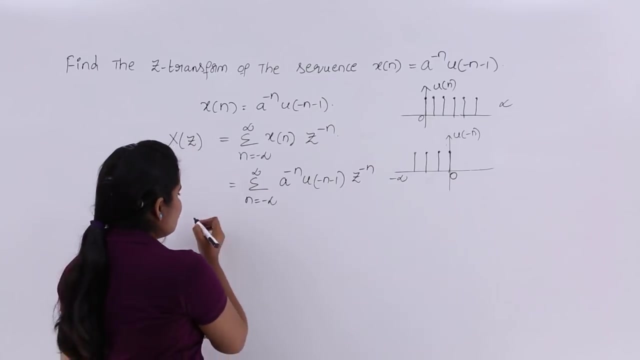 this. that means 0, 1 minus 1, 2, 3. this is u of minus n. so u of minus n is always from 0 to minus infinity. So here for u of minus n you are having a shift. Which shift means? that is a right shift, for example, for any signal x of n, if you are having 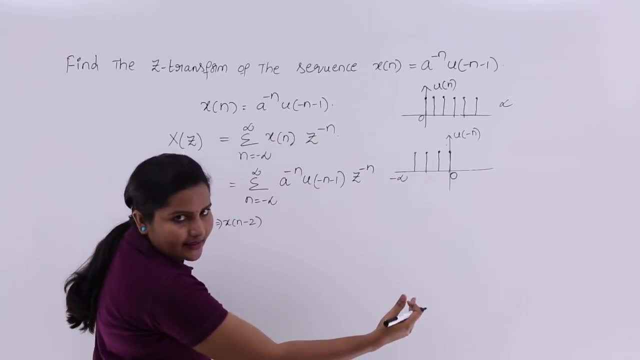 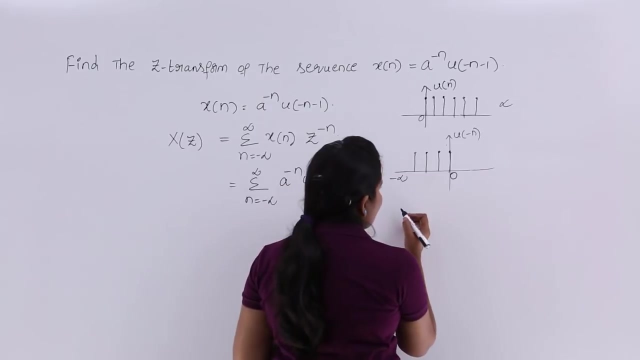 x of n minus 2, then that is called as right shift. if you are having x of n plus 2, that is called as left shift. but here forever u of minus n, you are having right shift. so that means if you are having minus 1 means you are having right shift. 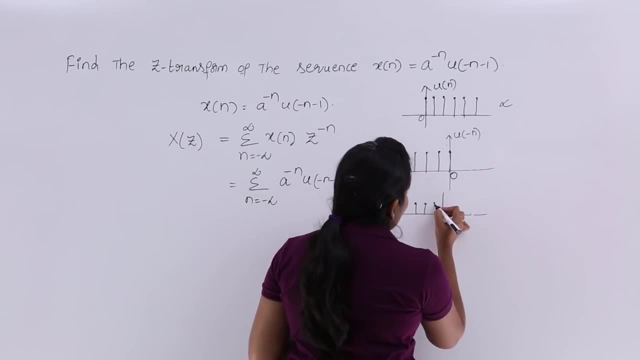 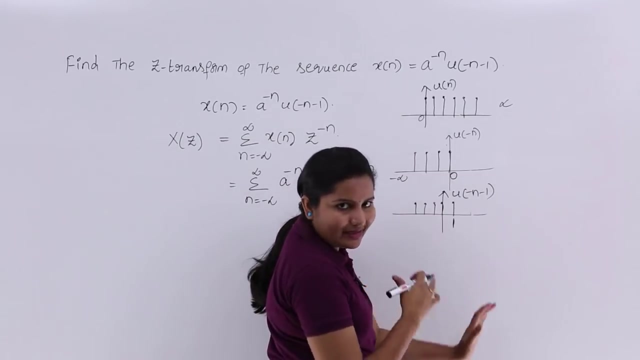 So your u of Minus n minus 1 signal will be like this: this is the signal of u of minus n minus 1. this is from so here up to 1 only. this is limited right side. this signal is limited up to 1. 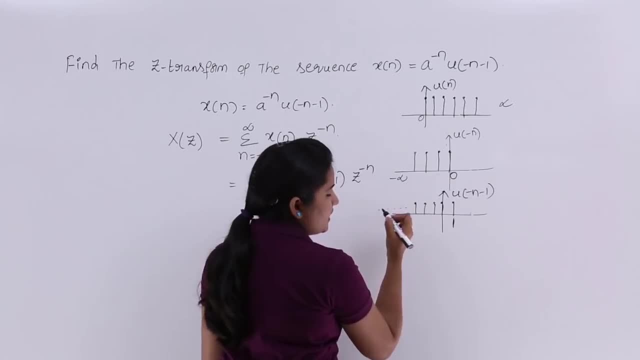 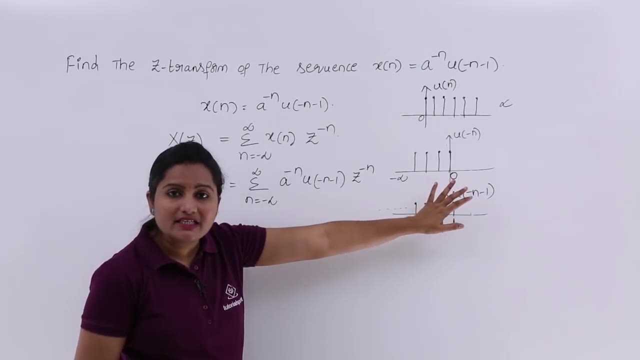 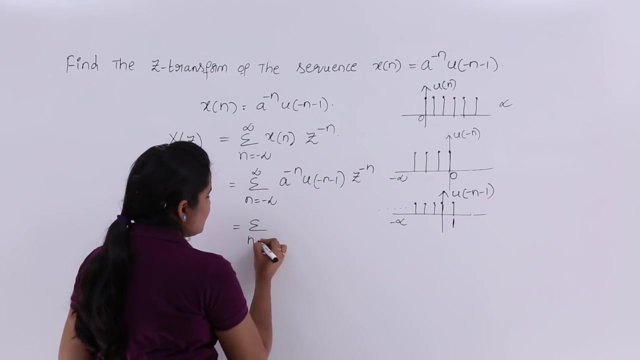 but left side keep on decreasing. that means keep on giving 1 up to minus infinity. So this signal region, the unit step signal region, is from minus infinity to 1.. So this is the signal region. So this will change the limits. means summation n is equivalent to minus infinity to 1, like 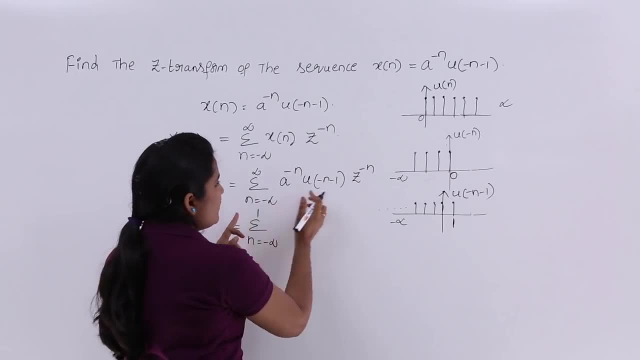 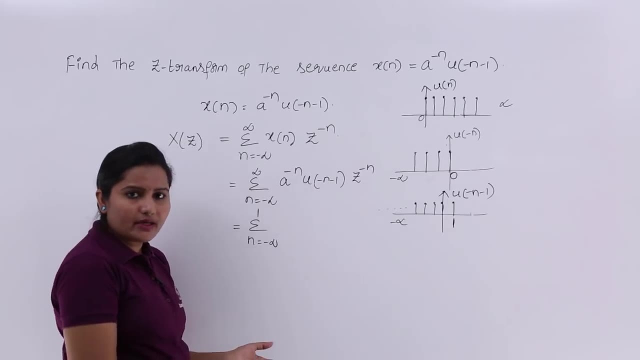 this it is going to limit. So minus infinity to 1, this value is equivalent to 1. now onwards, after changing the limits, no need to write that unit step function. why? because in this region that means from minus infinity to 1. this unit step function value is equivalent to 1. no need to multiply 1 every. 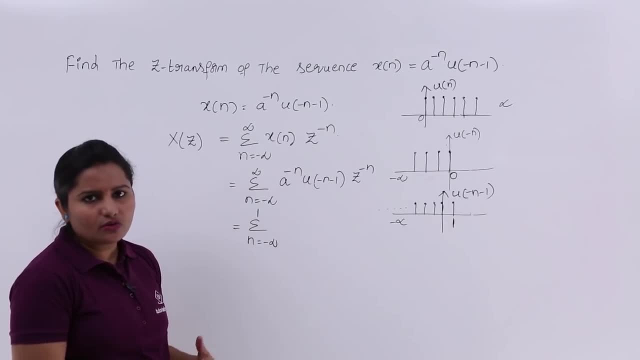 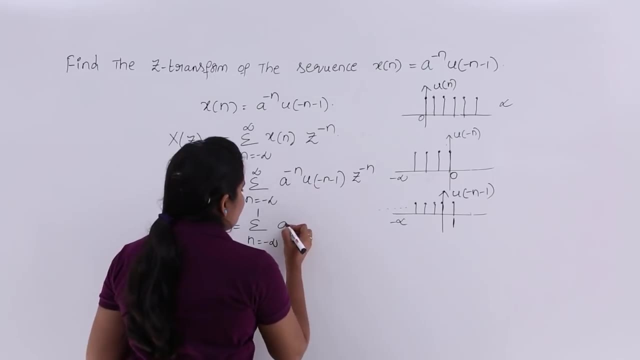 time You can neglect that. 1. Without neglecting that. 1. Without writing also no problem. but that effect we need to consider here in summation. So here: minus n z, power minus n- I am not writing u of minus n minus 1, because that value is. 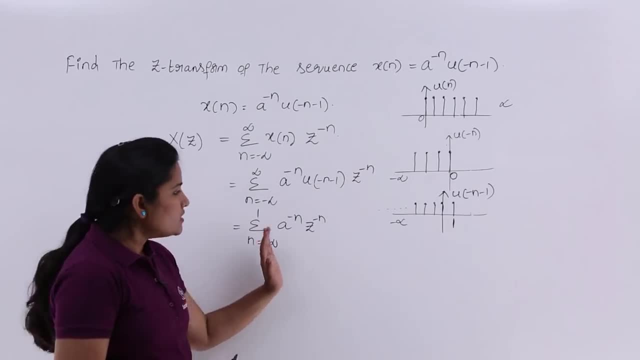 1, if you consider that 1 or not considering no problem. So now here you are having. n is equivalent to minus infinity to 1. a power minus n, z power minus n. So this is equivalent to summation, n equivalent to minus infinity to 1.. 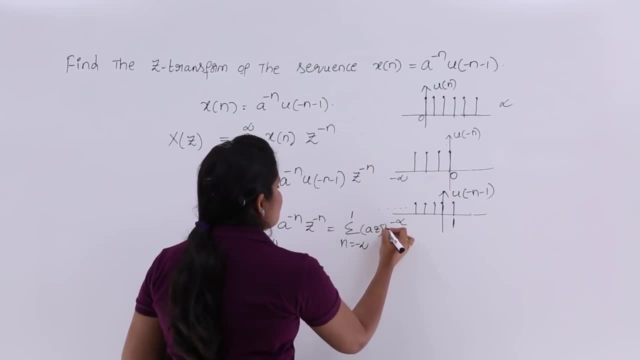 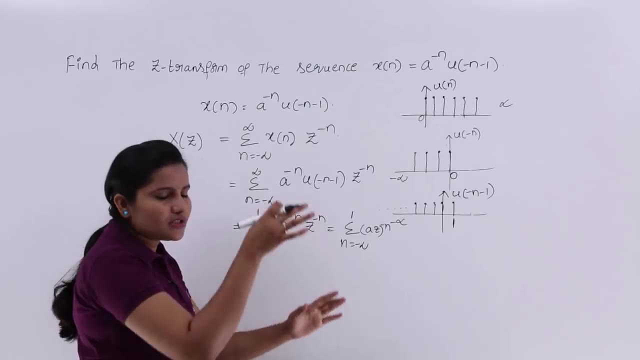 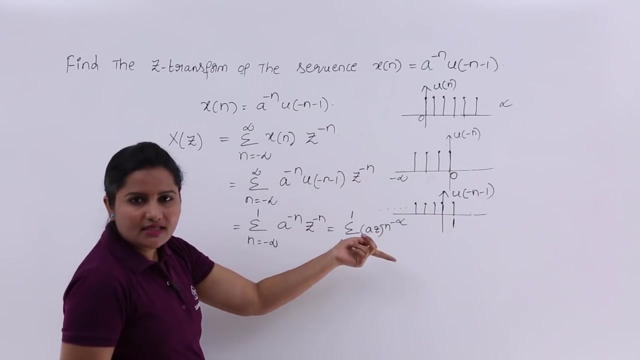 I am having a z whole power minus n. I am having a z whole power minus n. Here you can follow another procedure. if you want to reverse the limits of this summation, you need to write down the negative power. already negative power is there, so you can. 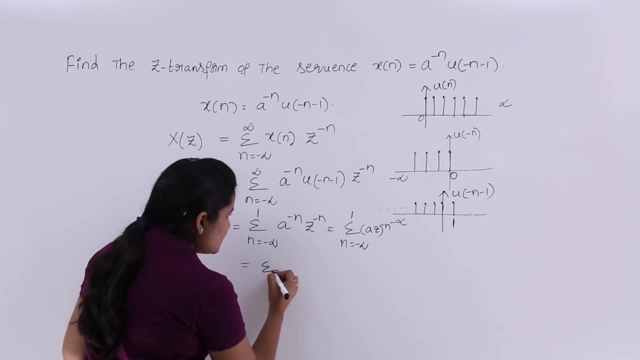 write the positive power. so you can also write like this: n is equivalent 1 to infinity. If you want to change the limit like this: a z whole power minus minus n, I am having a z whole power minus n. So you can write like that: 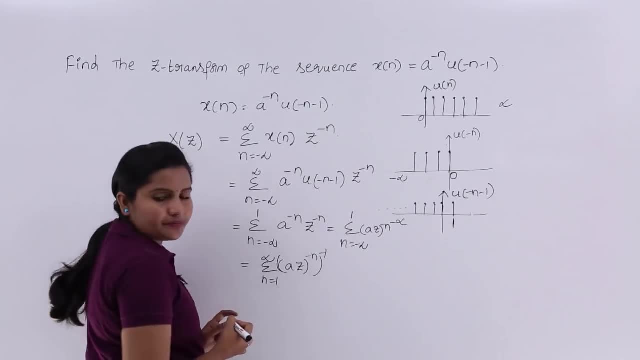 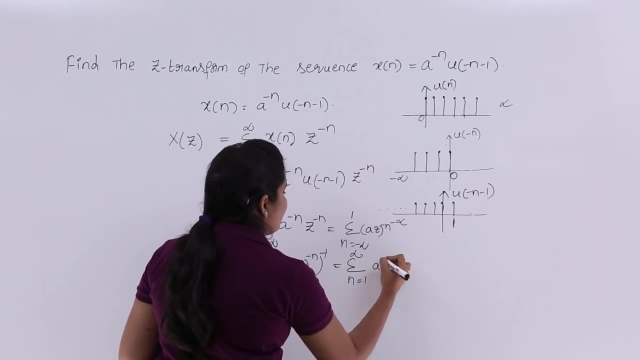 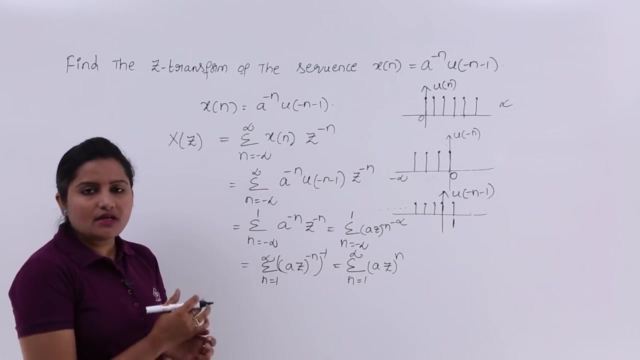 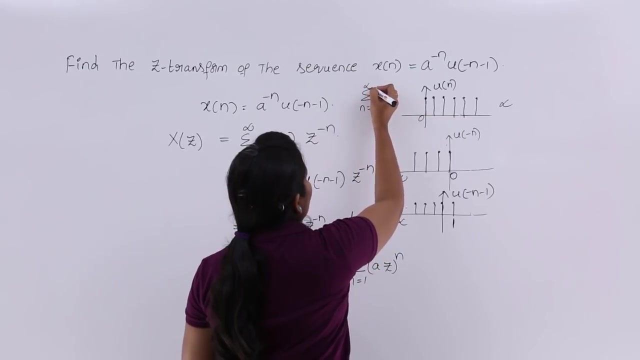 So this is equivalent to 1 into infinity n- whole inverse. you need to consider: Now this is equivalent to summation n is equivalent to 1 to infinity a, z whole power n. Now we are having equation for summation n equal to 0 to infinity a power n. for this I am having equation n equivalent to 0 to infinity if 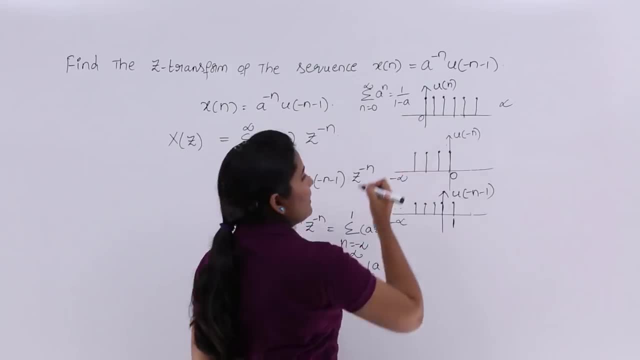 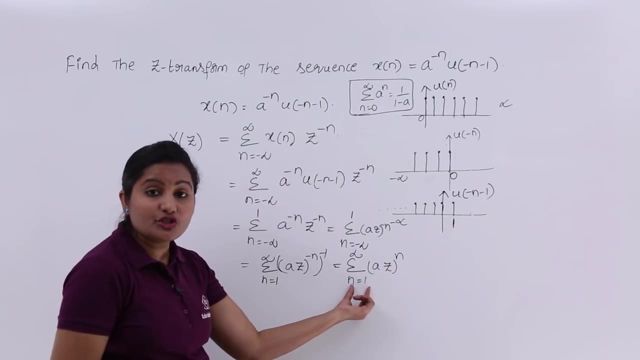 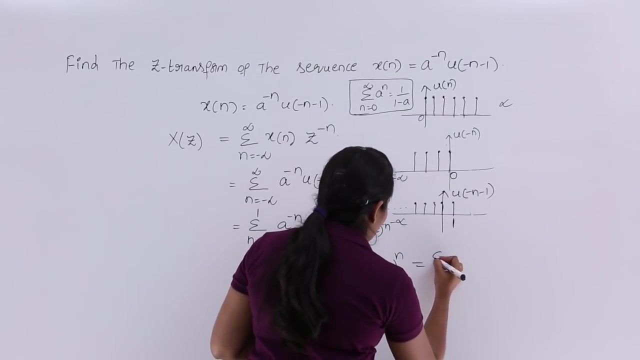 I am having a power n 1 by 1 minus a. I can write: This is a fundamental formula, but here I am not having from 0 to infinity, I am having from 1 to infinity. If I want to write like this, if I want to write this as n equal to 0 to infinity: a z whole. power 0 a z whole. 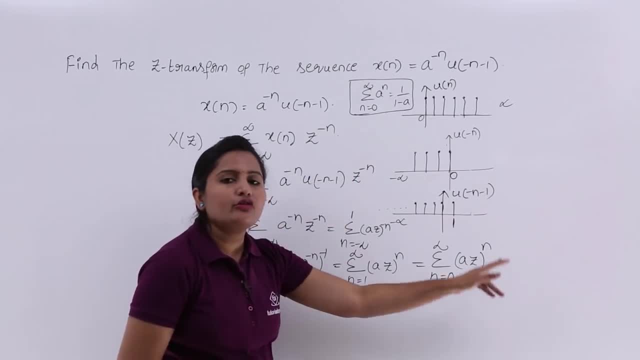 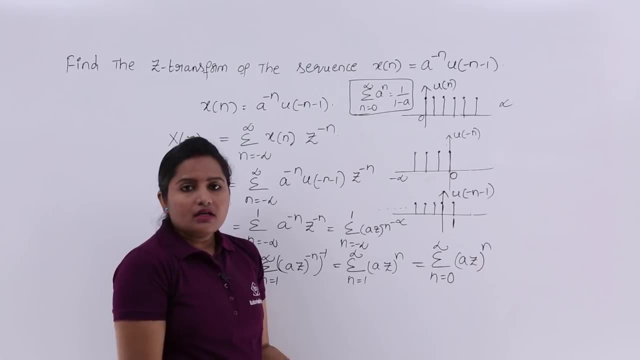 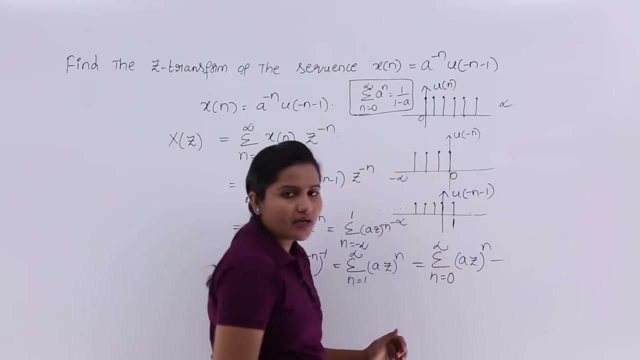 power n. this is the meaning I included. n is equal to 0, to infinity, a, z whole power. 0 is equivalent to 0 term in this summation, which is actually not there. So is it right? it is not right. whenever I am not including like this, I am writing: I included n equal. 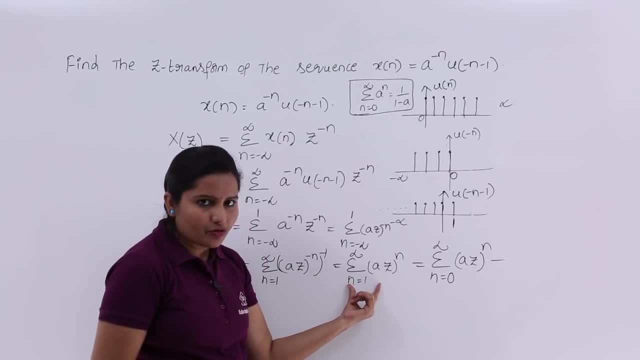 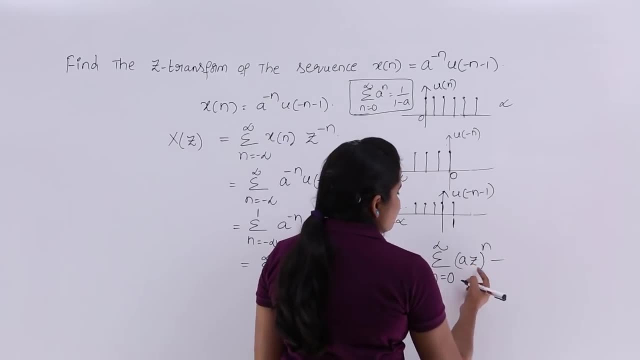 to 0 term. but that is actually not there in our process. that is why I am separating that, I am subtracting that, So n equal to 0. if I substitute, I am going to get a z whole power. 0 is equivalent to 1.. 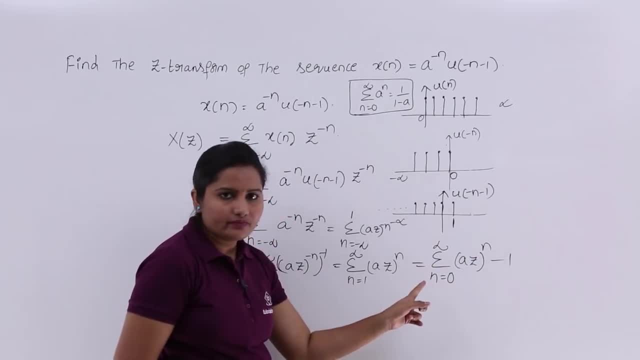 Now, if I written like this, I can write like this: If I want to write summation n equal to 0 to infinity, definitely I need to subtract that. whatever the term included in that summation, I need to subtract the term, otherwise I cannot include here. So now I written like this same thing. I written like this, I included. 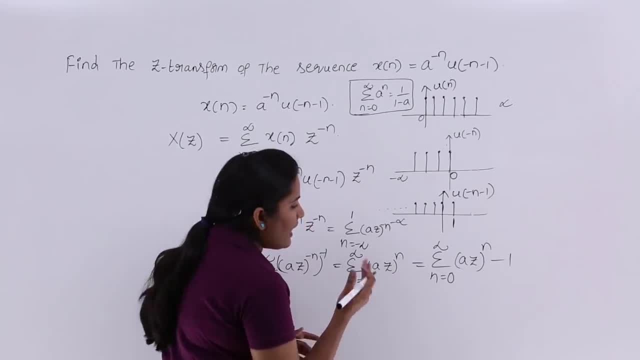 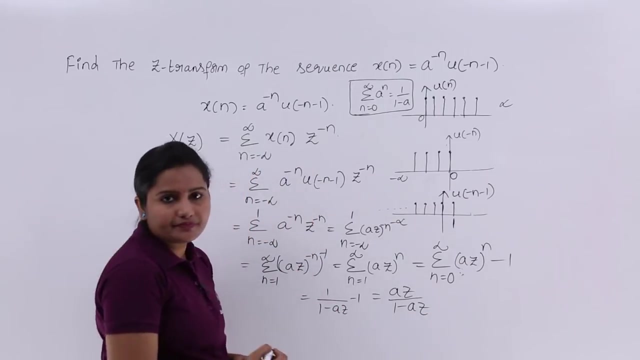 in summation and subtracted aside, and here now I am having equation for this. based on this So total term, if I consider like a, I can write 1 by 1 minus a z minus 1.. So this is equivalent to: if you done cross multiplication, So a z by 1 minus a z, you will get a z by 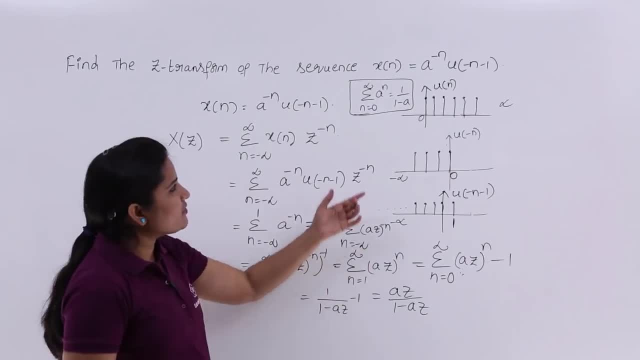 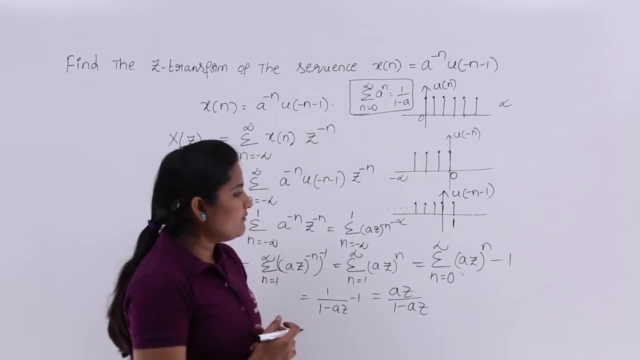 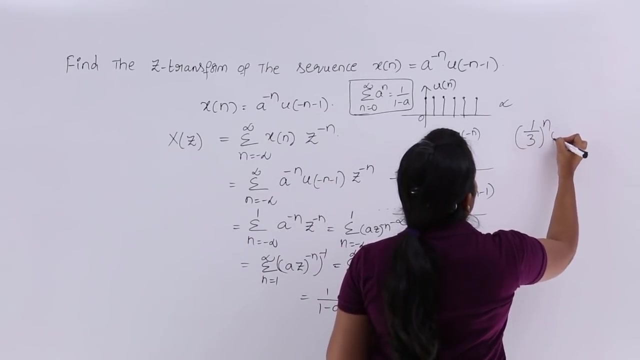 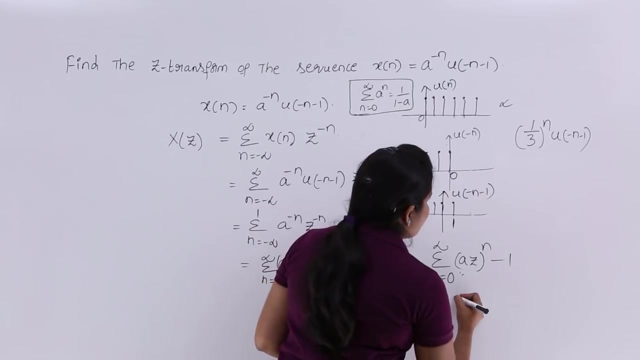 1 minus a z will be the z transform of the signal: a power minus n? u of minus n minus 1.. For example, if anyone given you like this, what is the z transform of 1 by 3? whole power n? u of minus n minus 1.. You can take this equation as I am writing once again: x. 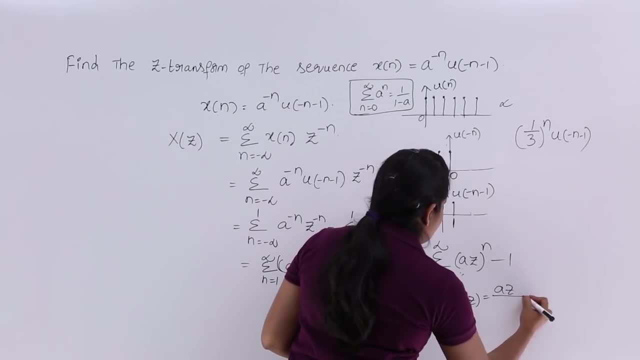 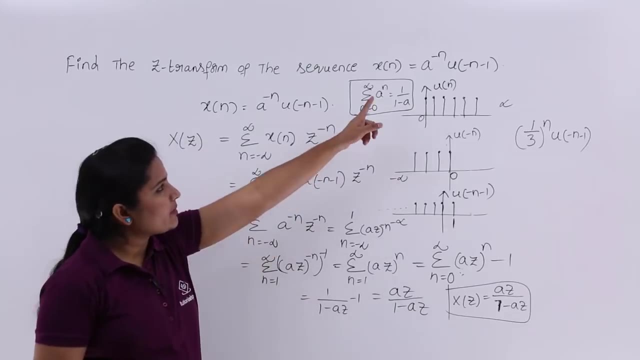 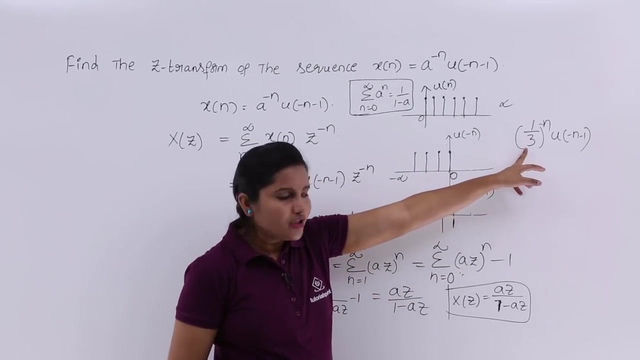 of z is equivalent to a z by z 1 minus a z. This is the transform of a power minus n? u, of minus n minus 1.. If you are having like this, if you given with this signal, you can, you can compare these. 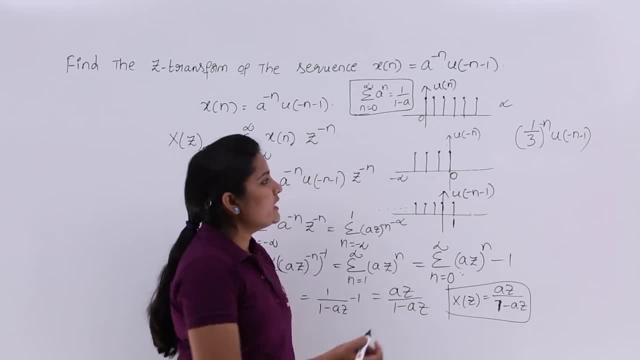 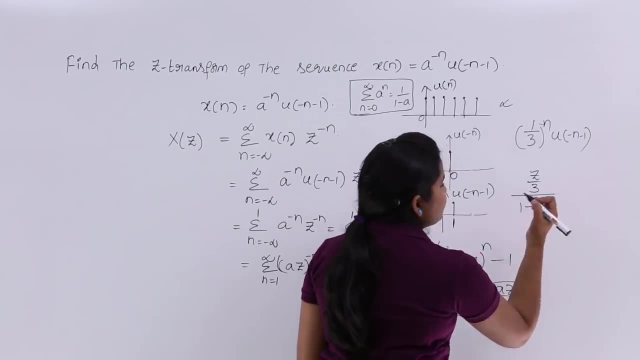 two signals and you can apply the same formula. That means in a place you are having 1 by 3.. So z by 3 divided by 1 minus z by 3.. So now, so z by so 3 minus z you are going to.